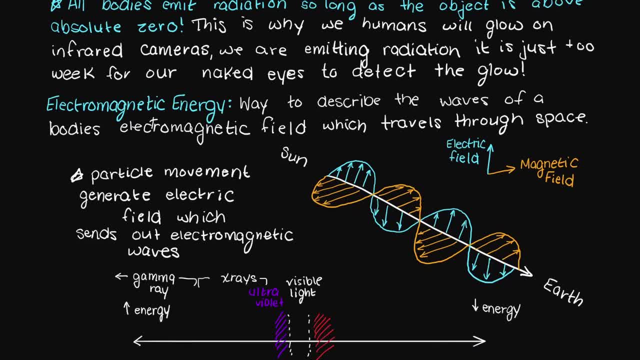 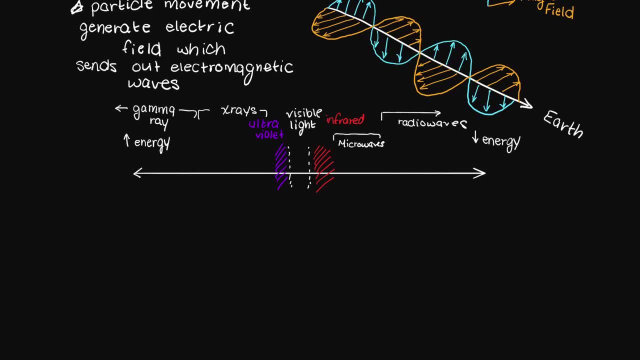 include radio waves, x-rays, ultraviolet rays, infrared, visible and gamma rays. As we have stated previously, all bodies above absolute zero will emit thermal radiation. Therefore, wouldn't everything be getting continually cooler if they are constantly giving away energy? Well, no, because bodies can also absorb energy from everything around it, as 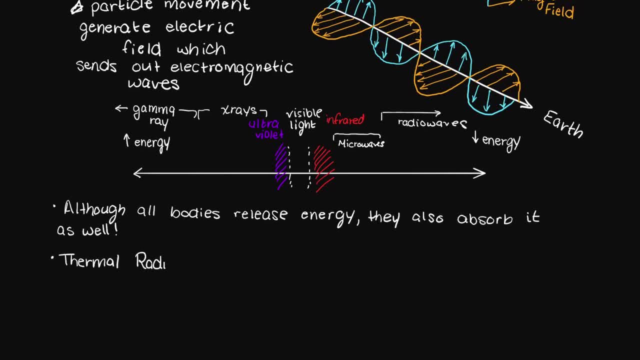 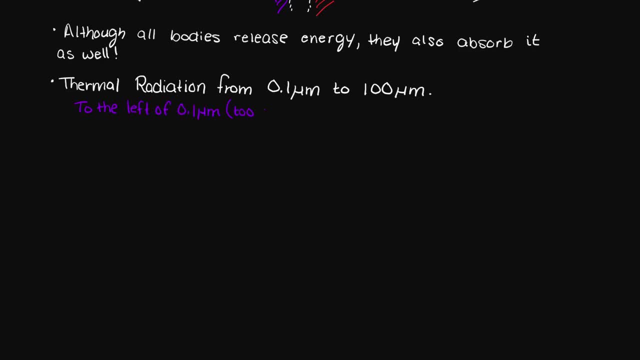 well, I just want to add that thermal radiation wavelengths are typically from 0.1 microns, which is in the ultraviolet range, to about 100 microns, which is in the infrared portion of the electromagnetic spectrum. To heat up many molecules in organic material, ie like 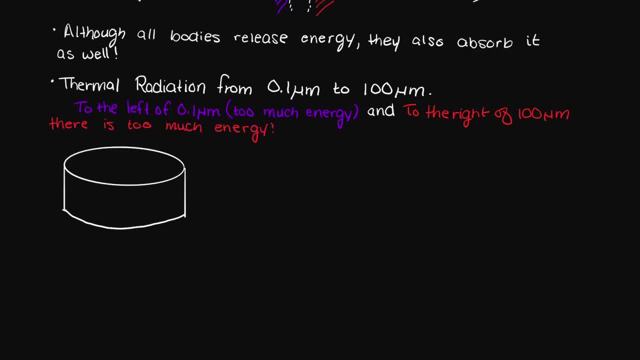 the water inside of us humans, the waves need to be at a certain frequency and energy. So at 0.1 microns there is simply too much energy, and to the right of 100 microns there is simply too little energy. I like to think of this as waves in a pool: If you splash your hand. 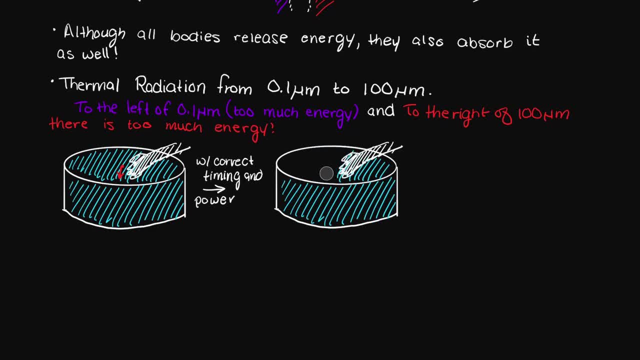 down. with enough force and time it correctly, you can get the waves bigger and more rhythmic. Now let's think of this like the particles in our body absorbing the energy as moving faster around us, therefore heating up better. However, if your hand is hitting too hard, 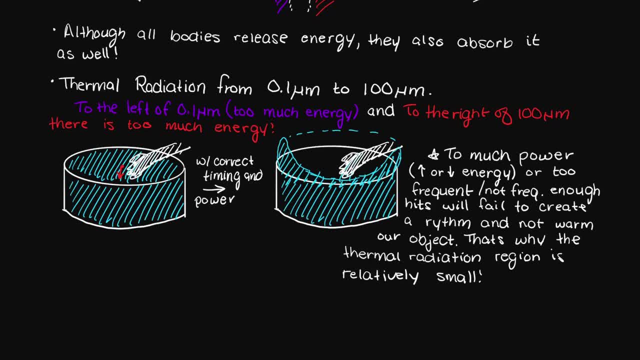 or too little or too fast or too slow, then you will have a hard time creating any decent waves in your pool. This is why thermal radiation is only considered over this certain region of wavelengths on the electromagnetic spectrum. We will talk more about the electromagnetic spectrum and 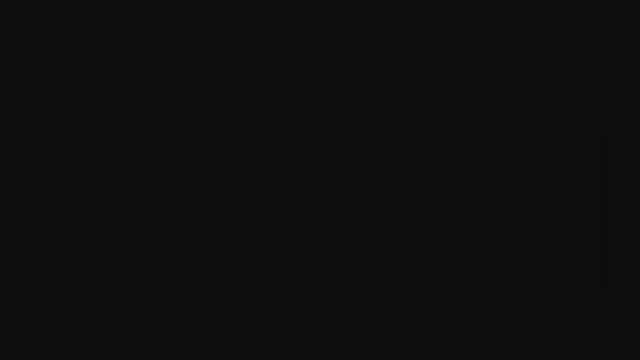 wavelengths more in the next video. So now that we have a rough understanding of what thermal radiation is, do you think that a body's temperature will affect how much energy is emitted from it? Well, of course, we have all experienced this. If you put your hand anywhere remotely close, 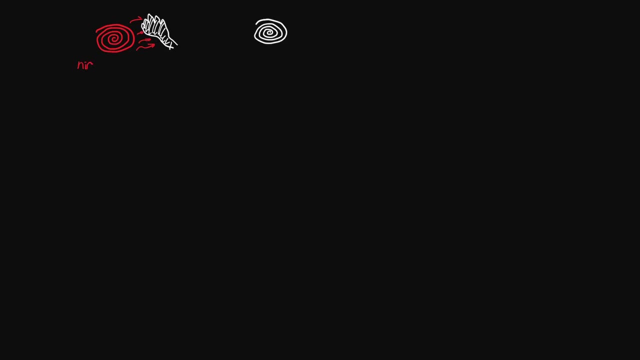 to a stove burner. while it is on, you will feel the energy radiating from the coils. However, if the stove burner is off, you will no longer be able to feel the radiating energy, even though it is still occurring. This is because, as we heat up the burner, there is much more. 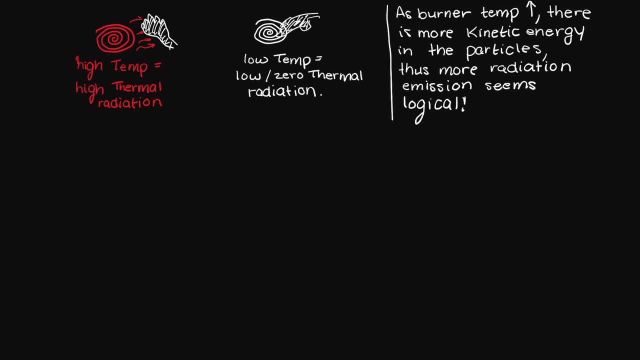 kinetic energy within the particles that can be converted and turned into thermal radiation, which is essentially the conversion of kinetic energy into electromagnetic energy. Thank you for checking out this video and I hope it helped you gain a broad understanding of thermal radiation. In the next video I will be going through the properties of thermal 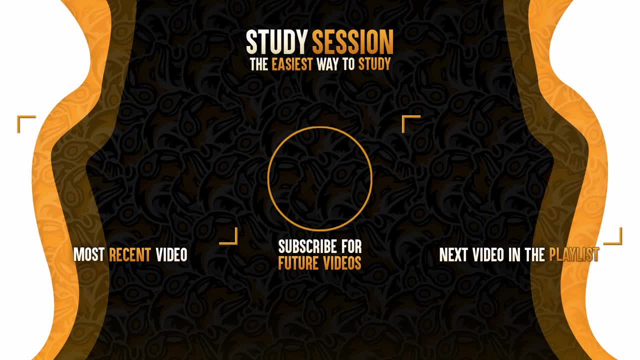 radiation. If you enjoyed, please like and subscribe to support the channel. However, if you have any comments or suggestions, please let me know in the comments below. If you have any comments, questions or concerns about the information I provided in this video. please leave a comment down below and I will do my best to address your concerns. 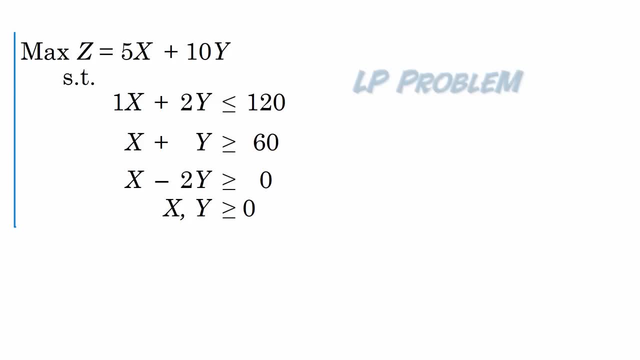 Welcome. In this tutorial, I will solve this LP problem using graphical approach and use it to explain the special case of alternative or multiple optimal solutions. Let's begin by finding points for drawing the constraint lines. For the first constraint line, when x is 0,. 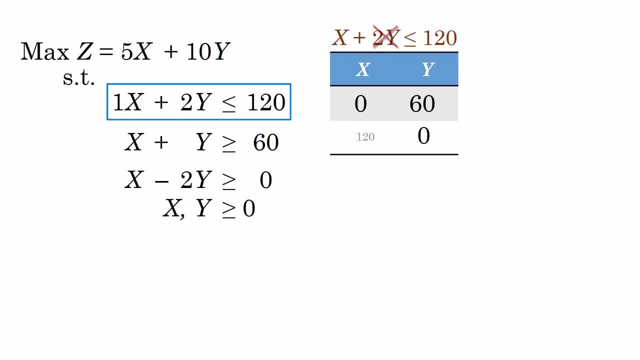 y is 60, and when y is 0,, x is 120.. For the second, when x is 0,, y is 60, and when y is 0, x is also 60.. For the third, when x is 0, y is also 0. 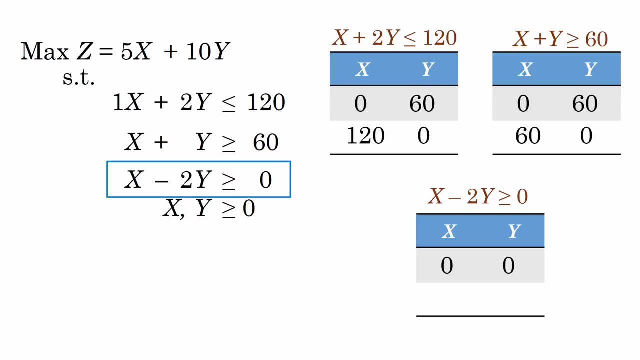 So to find another point, we can rewrite the inequality as x greater or equal to 2y. We can then pick a reasonable value for either x or y and calculate the other. For instance, if y is 50, x is 2 times 50, which gives 100. 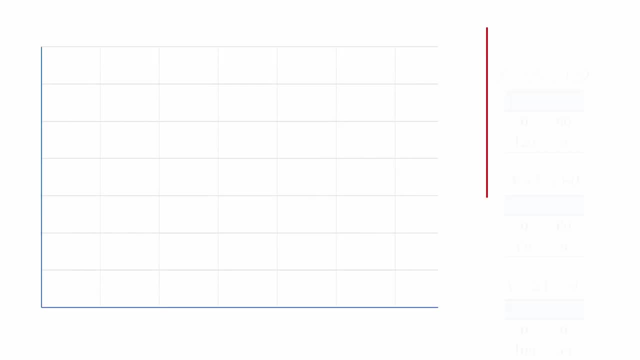 Let's now draw the graph. Here are the constraints, along with the x- y coordinate pairs obtained earlier. Since the highest x value we have here is 120, and the highest y is 60,, we can go up to 120 on the x-axis and up to 60 on the y-axis. 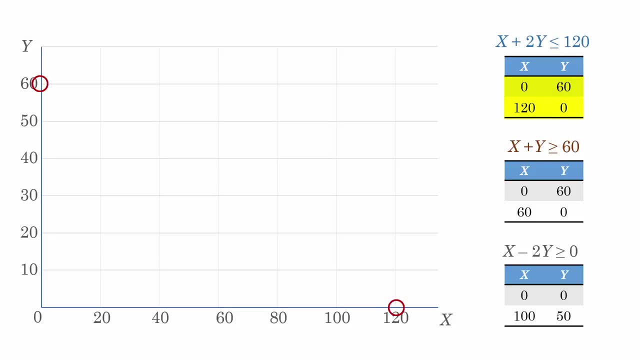 For the first constraint, we have 0, 60 and 120, 0.. We join the points for the constraint line And the two constraints. we have a point at 0, 0 and another at 150.. For the second, we have 0, 60 and 60, 0.. That's the line.